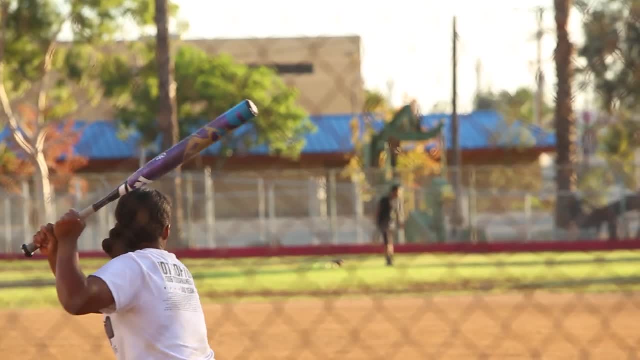 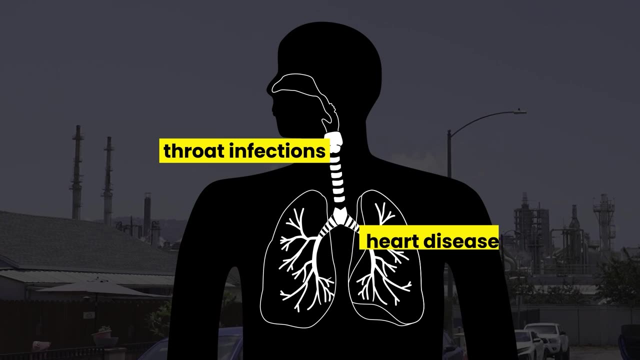 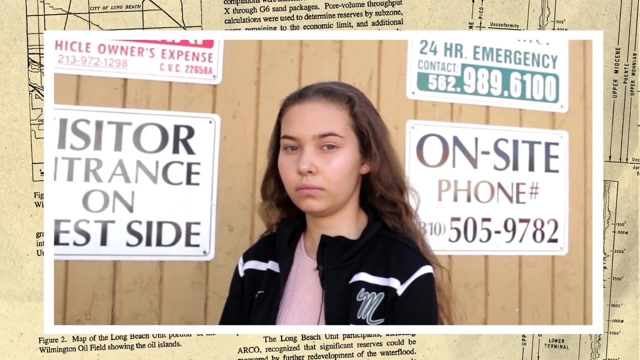 and are inhaled by people living, working or playing nearby. Living near oil operations is associated with high rates of throat infections, heart disease, asthma, cancer and miscarriages. Teenagers living in Wilmington shared their experiences of living close to oil wells. 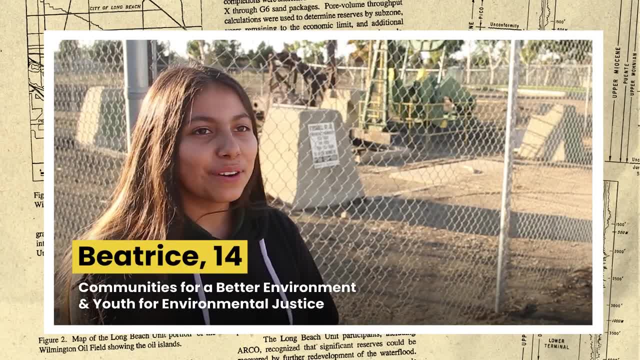 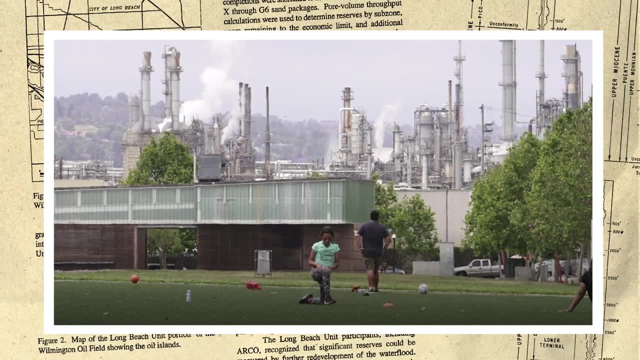 I live close to an oil well- It's like a couple feet away- And I really care about my family because I have a sister that has a heart problem. If it's too hot she throws up a lot. If it's cold, her lips turn purple, blue or something like that. 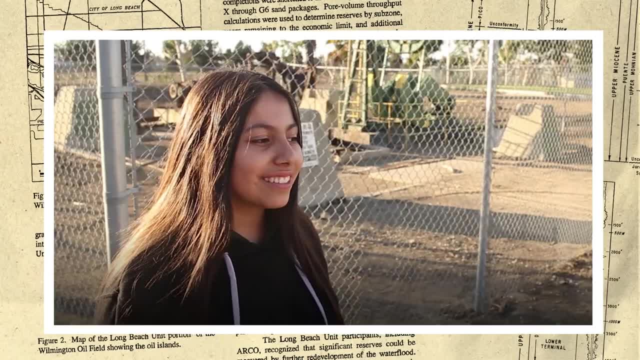 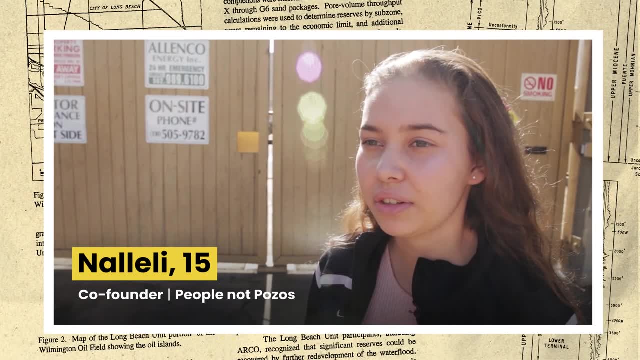 So we have to really take care of her. These aren't normal for your community. I suffered from heart palpitations. I had to use a heart monitor for several weeks. I had body spasms that got to the point where I couldn't walk. 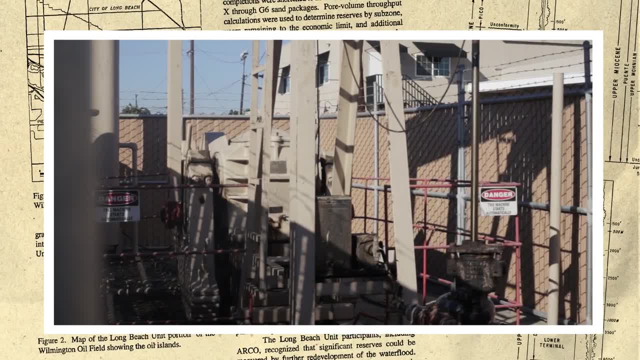 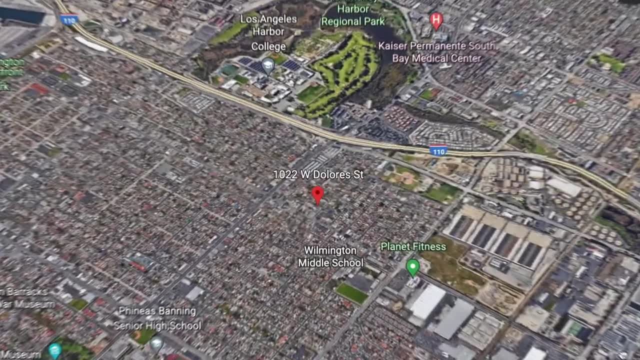 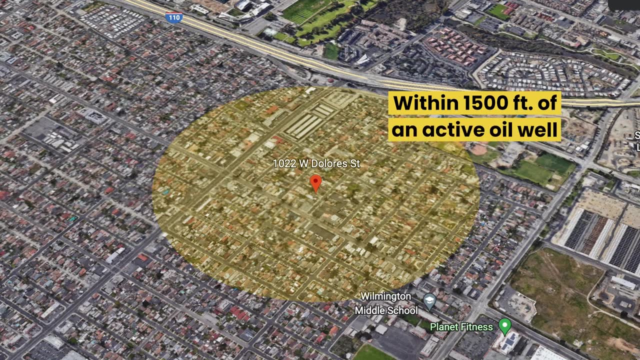 There's nothing else to do but shut it all down. These oil wells shouldn't be here in the community, around schools, around churches, around residential facilities. In 2017, UCLA conducted a household survey with residents living within 1,500 feet of. 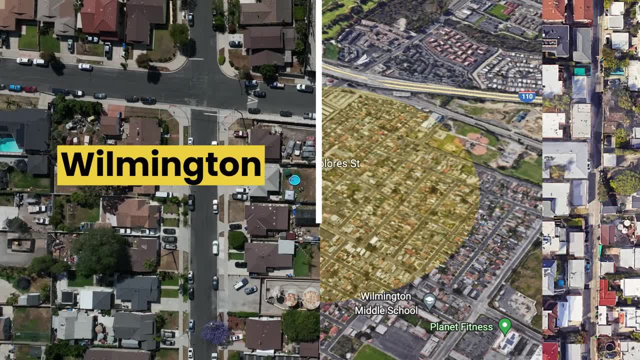 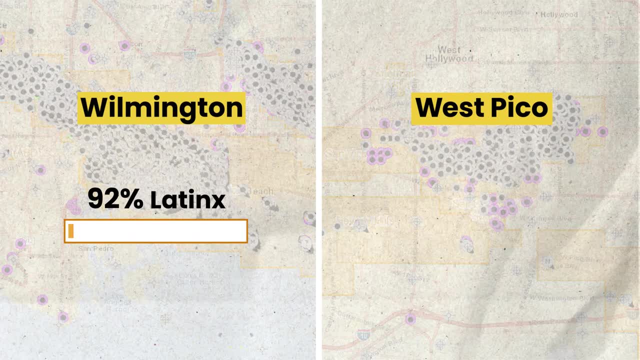 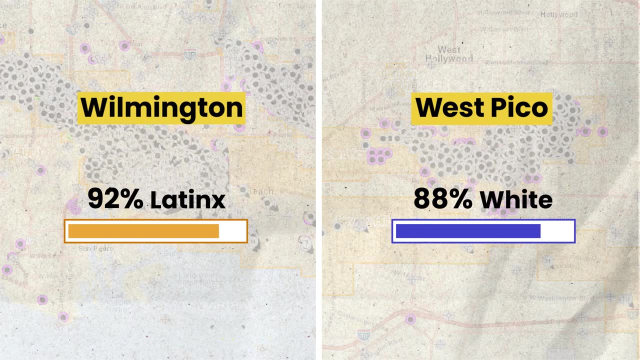 an active oil well in the neighborhoods of Wilmington and West Pico. Both neighborhoods have oil wells scattered throughout the community. We found that 92% of Wilmington residents were Latinx and 88% of West Pico residents were White. When asked whether they felt safe from pollution, only 2 out of 10 Wilmington residents felt. 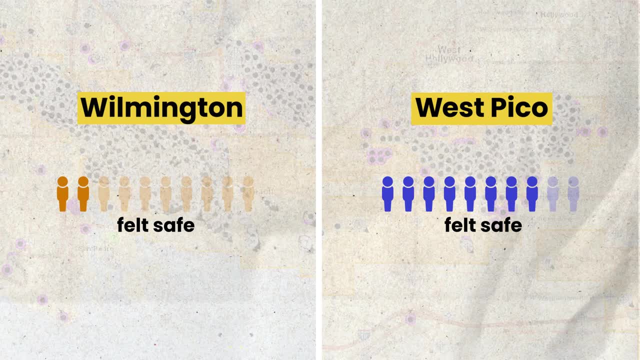 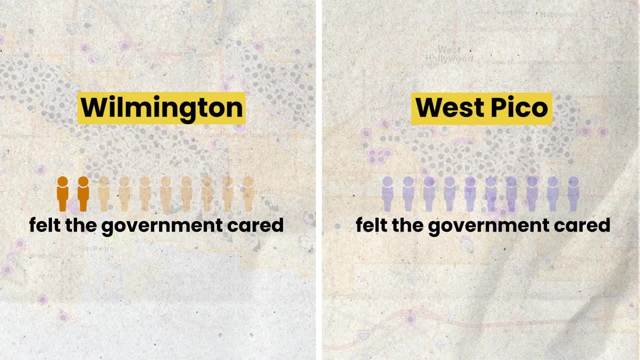 safe. while 8 out of 10 West Pico residents felt safe When asked whether they felt the government cared about the well-being of their community, only 5 out of 10 Wilmington residents felt the local government cared, while 9 out of. 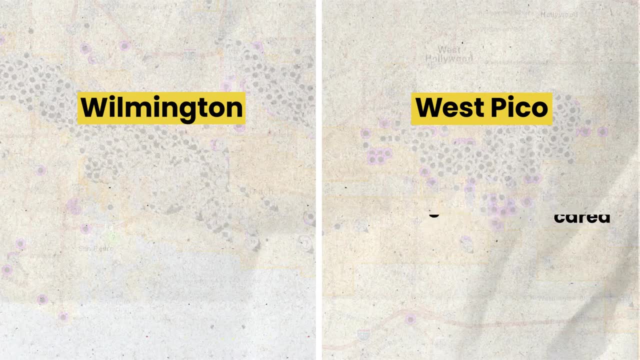 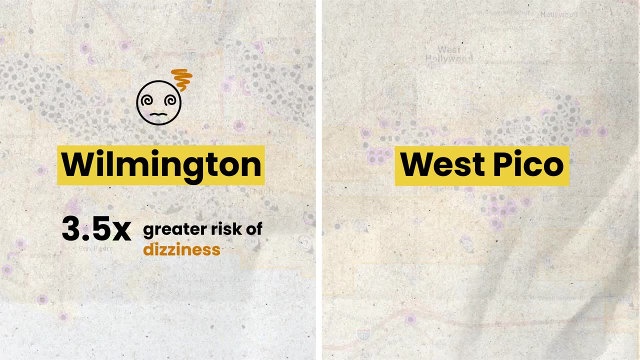 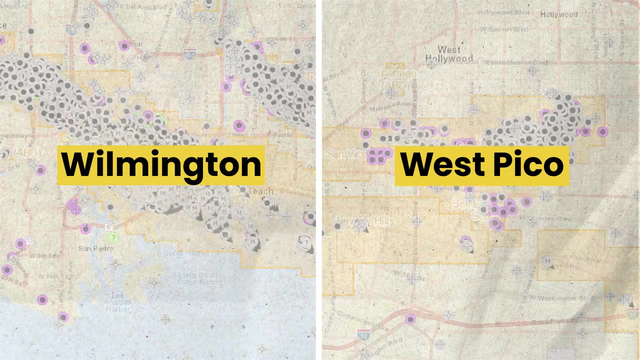 10 West Pico residents felt the government cared. Compared to West Pico, Wilmington residents reported significantly higher rates of nausea, dizziness, throat infections, chest pain and heart disease. Why might two communities that both have active oil wells have such different opinions and 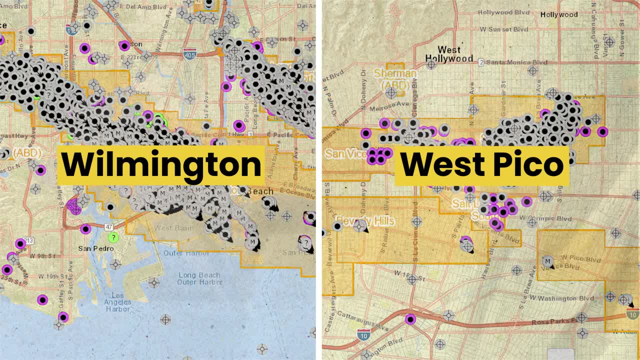 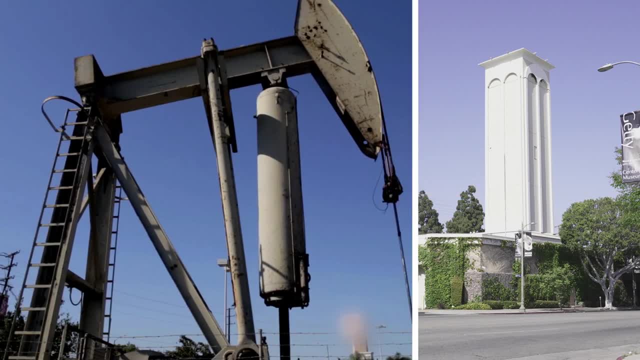 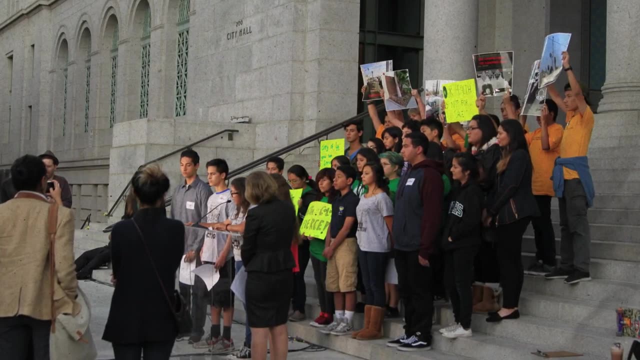 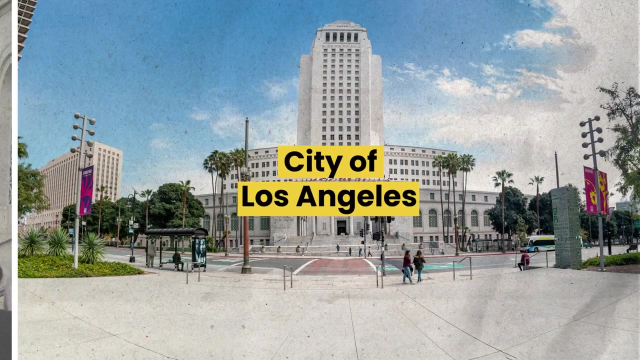 health outcomes. The answer is environmental injustice. Weaker enforcement of environmental regulations within a Latinx community is racial discrimination. To fight this, teenagers in Wilmington and South Central LA organized with their communities in 2015 to file a lawsuit against the City of Los Angeles. 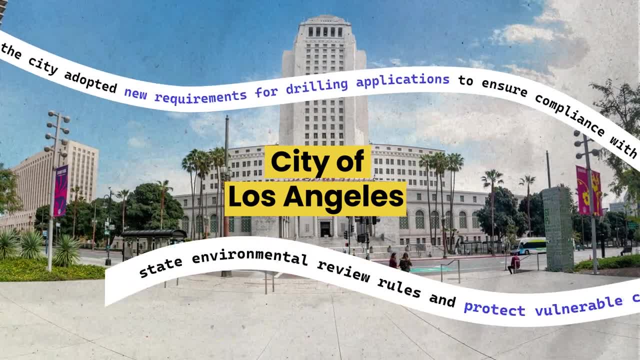 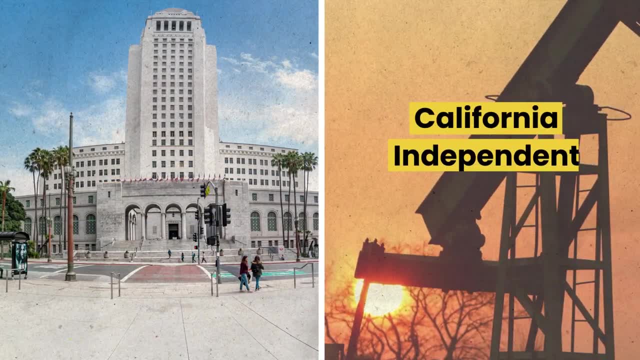 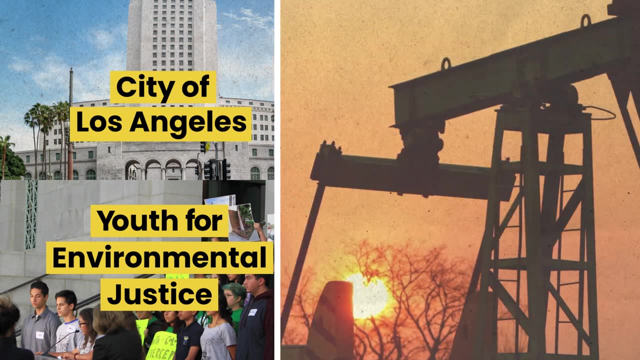 To the city's credit, the City of LA listened to these teenagers and changed its requirements for drilling applications, But…. The California Independent Petroleum Association counter-sued the city and the teenagers. In the end, the courts dismissed the oil industry's lawsuit and ordered it to pay over two million. 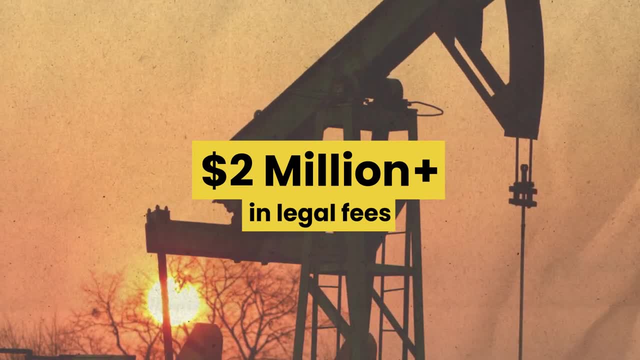 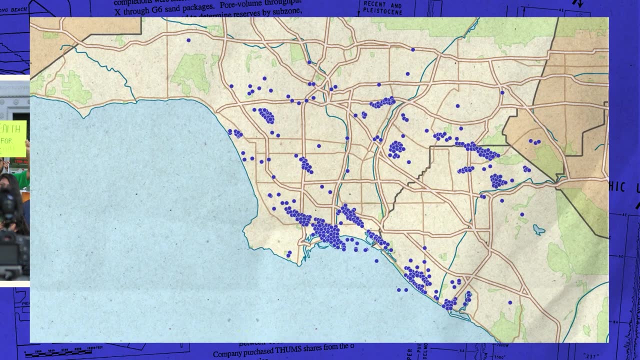 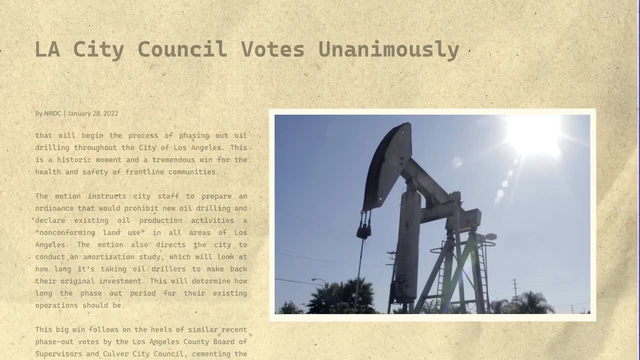 dollars in legal fees to the city and the lawyers who defended these teenagers. These teens triumphed. The ultimate goal of environmental justice is to prevent environmental harm for all communities. That's why it was such a big win when the LA City Council unanimously approved the 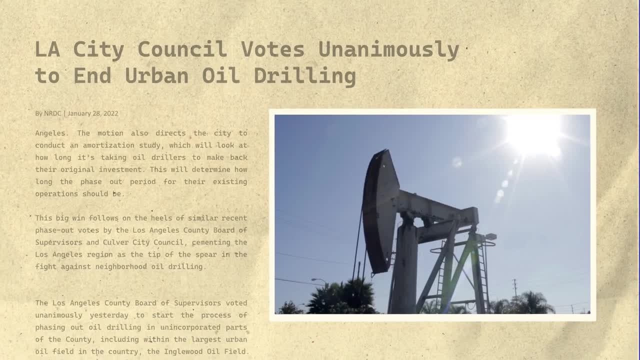 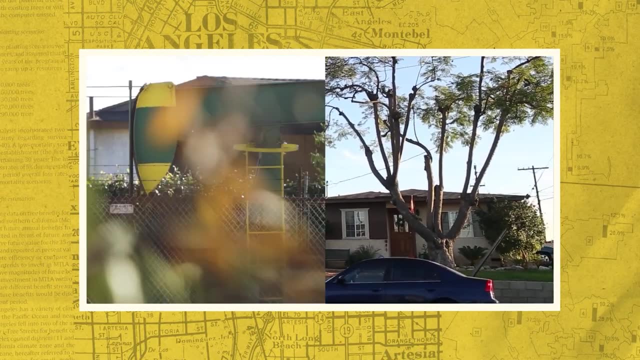 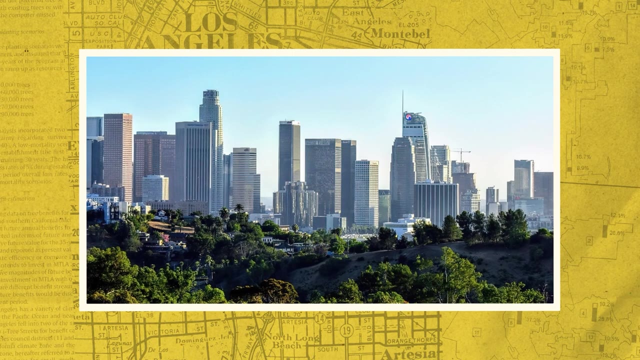 bill to end oil drilling in the City of LA. These teens won their fight and contributed to the surge of support to end neighborhood oil drilling in Los Angeles. But their case is one of many. Environmental justice is about ensuring we all have access to clean air, clean water. 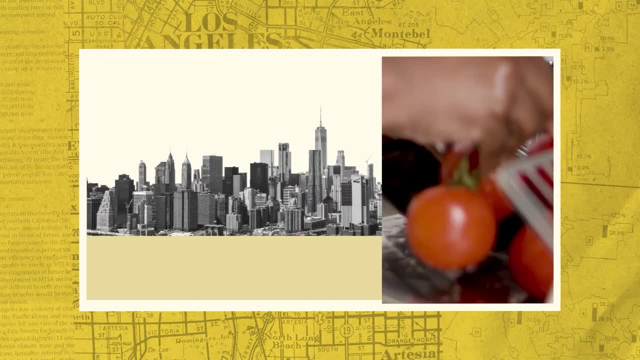 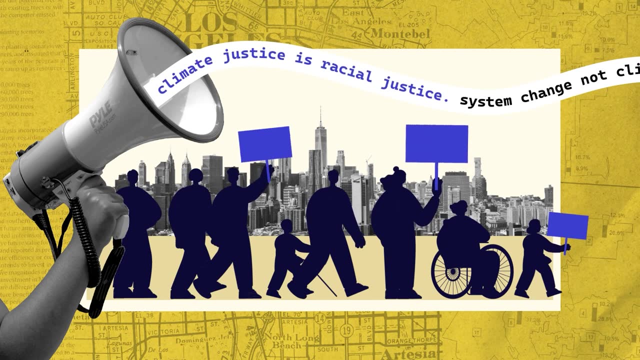 safe homes and nutritious food, And strengthening environmental justice means leveling the playing field. And strengthening environmental justice means leveling the playing field. And strengthening environmental justice means leveling the playing field So that all people can have a voice and influence in the decisions that impact them. 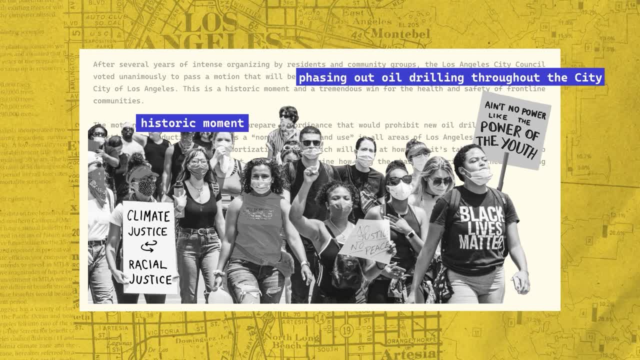 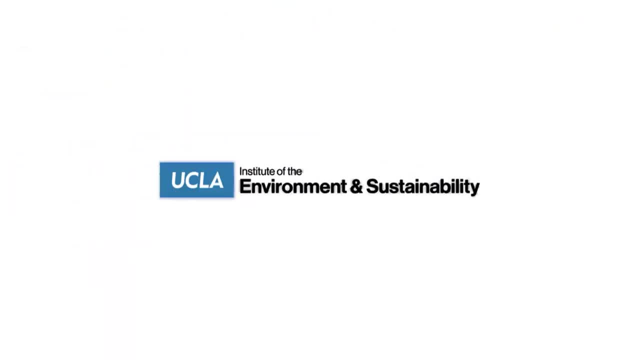 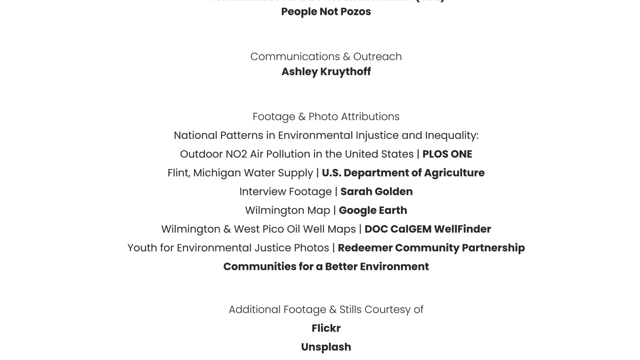 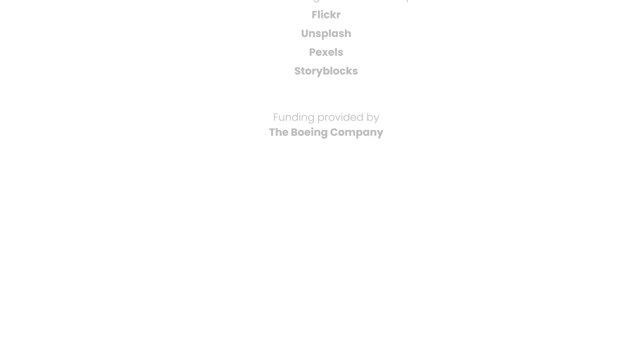 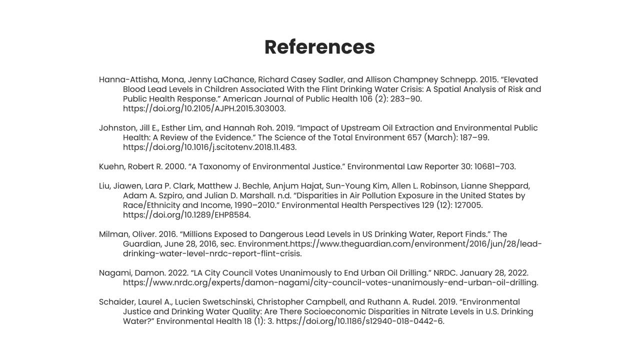 We can all have a voice. Use your voice to fight for a greener and more equitable future. Thank you, Thank you.